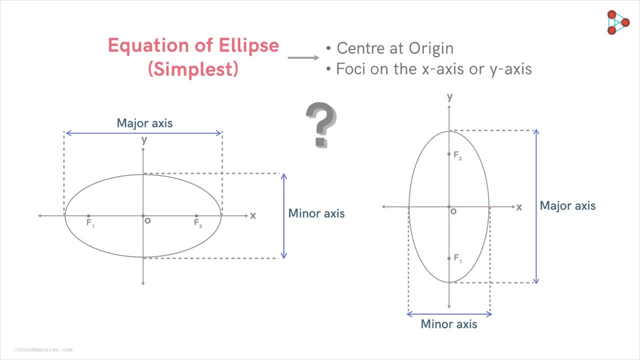 axis, along the x-axis. Will there be any more possible orientations of an ellipse satisfying these conditions? No, These two are the only two possible orientations satisfying these conditions, So we will only consider these two orientations. Let's first find the equation of an ellipse. 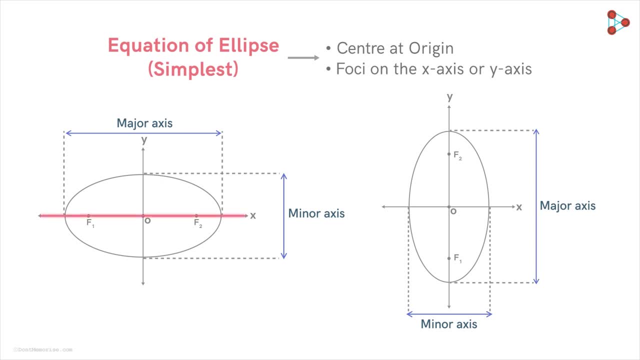 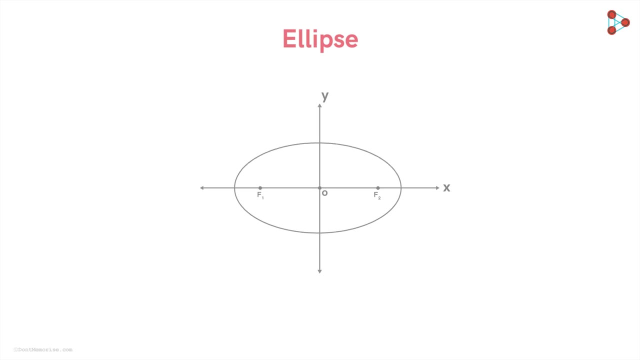 for this orientation with the foci on the x-axis? Tell me until now. what do we know about an ellipse? Yes, We know that for any point on the ellipse, its sum of distances from the foci is constant. Do you know what will be the value of this constant? 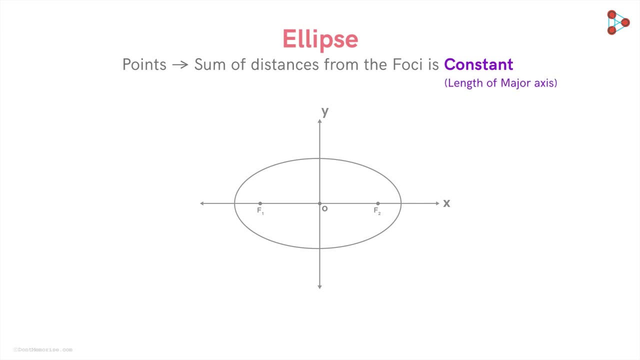 It turns out that this constant will be equal to the length of the major axis. How, Let's see. Let the length of the semi-major axis be A, and also let the distance between the centre and the focus of the ellipse be C. Now consider this point Q at one end of the major axis. What will be its sum of distances? 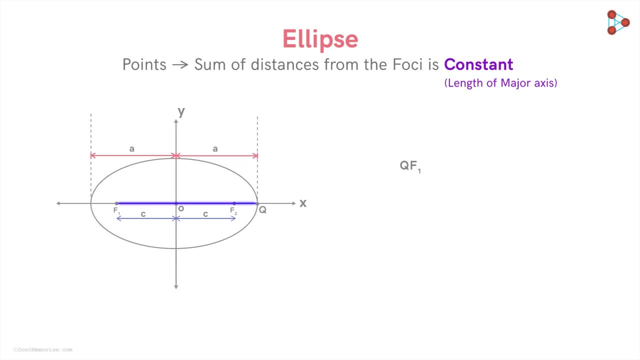 from the foci. It will be the sum of this distance, QF1., Which will be C plus A, And this distance, QF2., Which will be equal to A minus C. So we get this. We can see that this sum is equal to 2 times A. 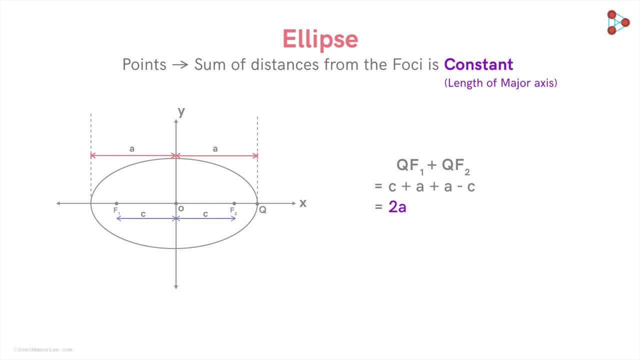 And we know that for any point on the ellipse, its sum of distances from the foci will be this constant 2A, And 2A is the length of the major axis of the ellipse. So we see that for all the points on the ellipse, the constant sum of distances from 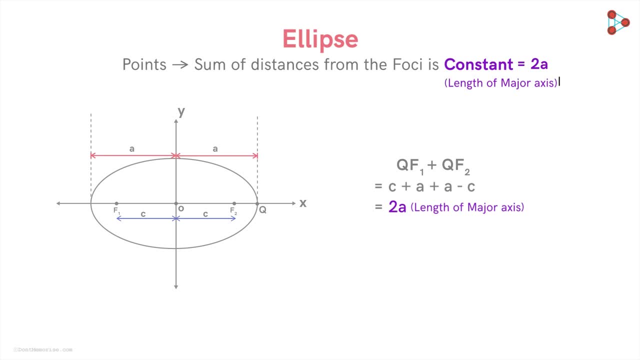 from the foci is equal to 2A, which is the length of the major axis. We discovered one more thing about the ellipse in the previous video. There is a relationship between the semi-major axis, the semi-minor axis and the distance from the centre. 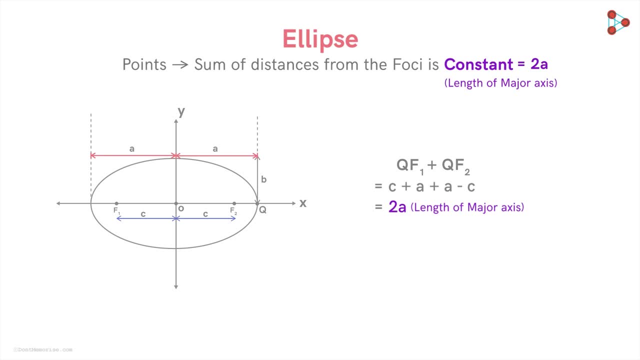 of the ellipse to the focus of the ellipse. Now, if we take the length of the semi-minor axis as B, then this is the relationship we saw earlier. So these are the two major things we know about an ellipse. Let's use them to find its equation.